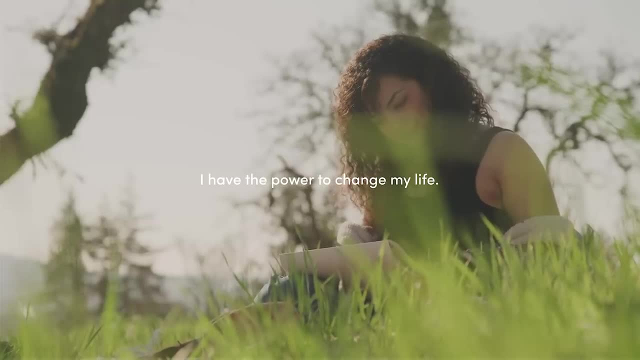 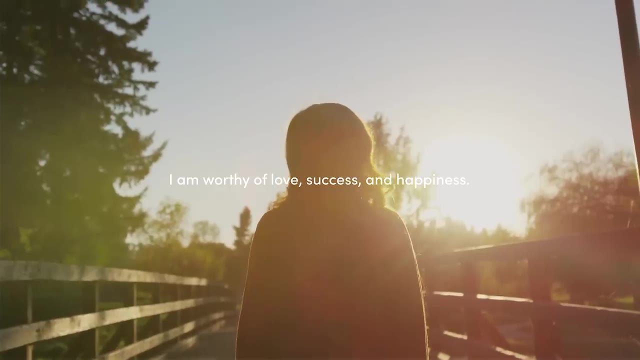 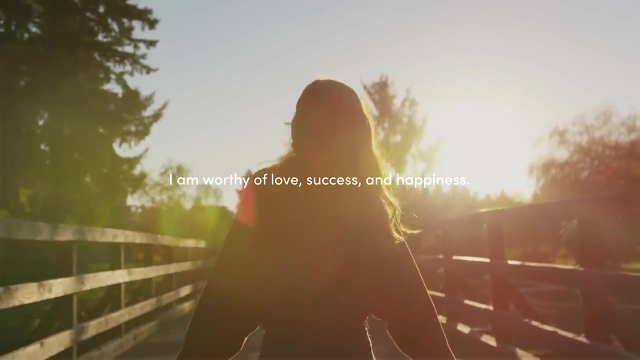 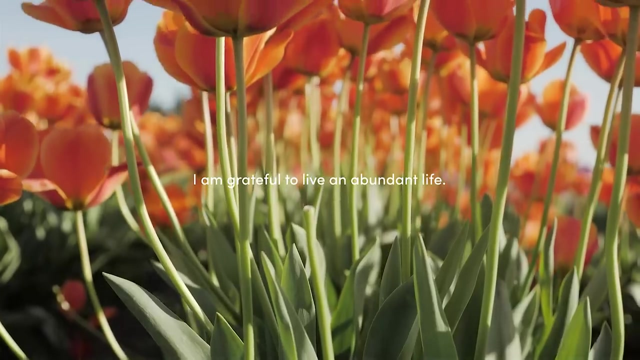 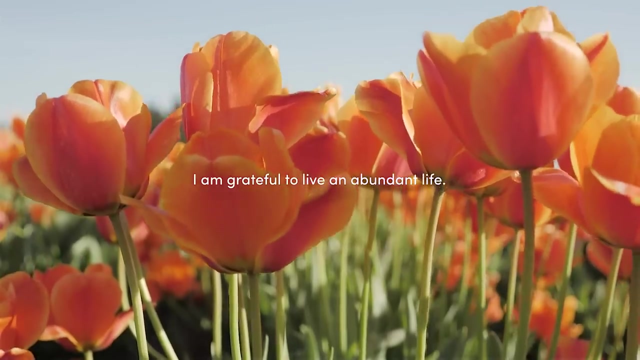 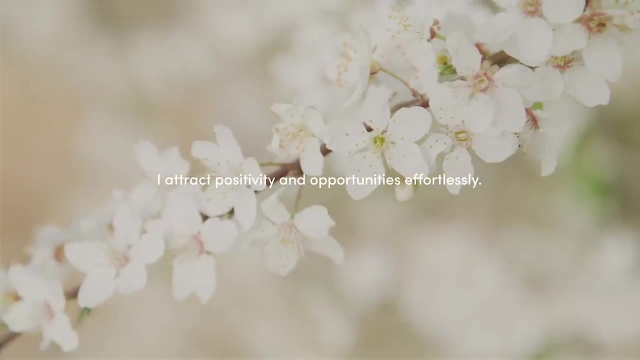 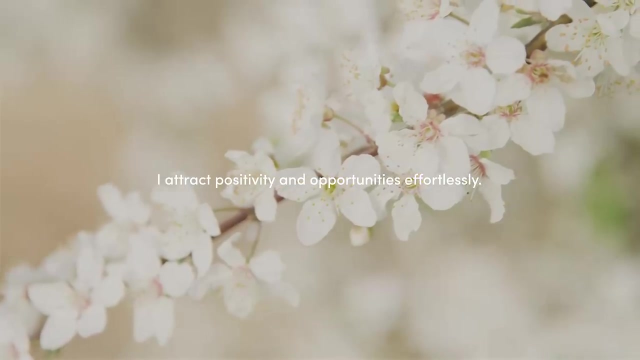 I have the power to change my life. I am worthy of love, success and happiness. I am worthy of love, success and happiness. I am grateful to live an abundant life. I am enjoying my life with and opportunities effortlessly. I attract positivity and opportunities effortlessly. 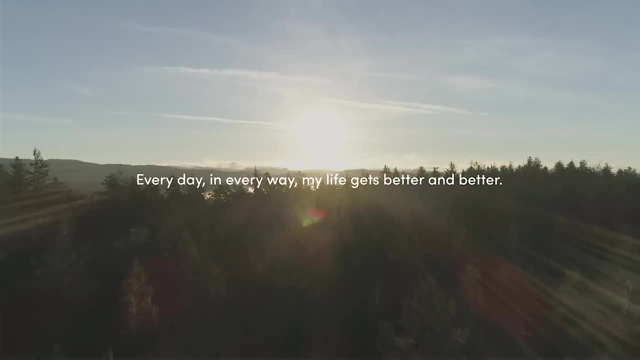 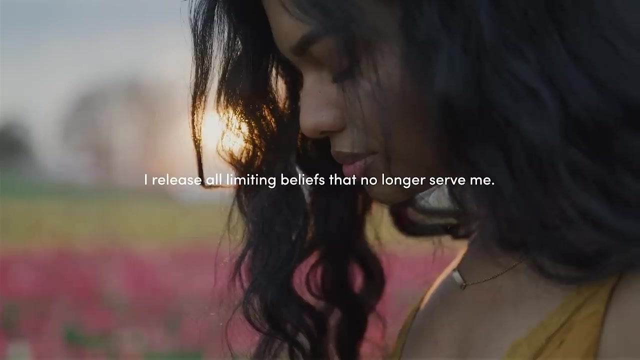 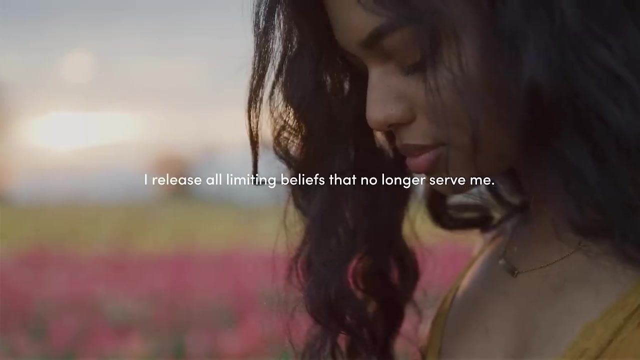 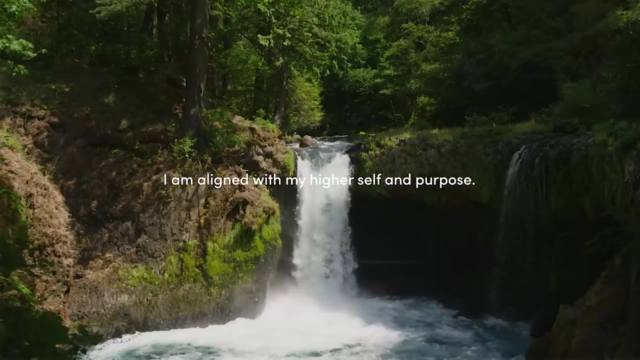 Every day, in every way, my life gets better and better. Every day, in every way, my life gets better and better. I release all limiting beliefs that no longer serve me. I release all limiting beliefs that no longer serve me. I am aligned with my higher self and purpose. I am aligned with my higher 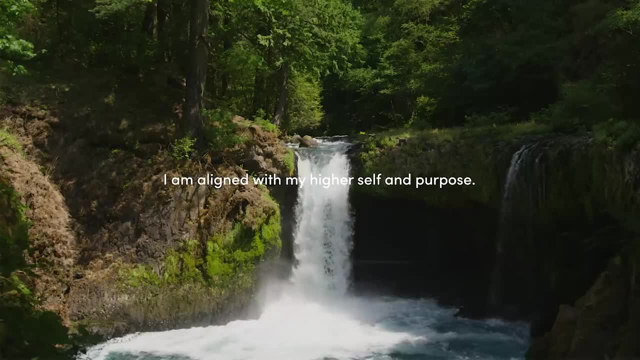 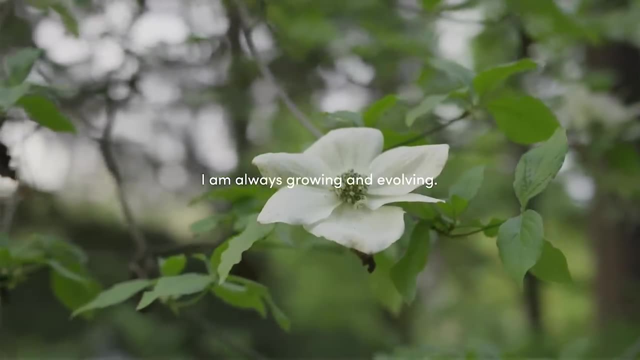 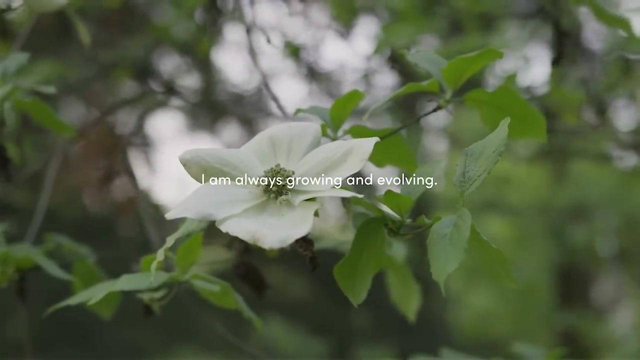 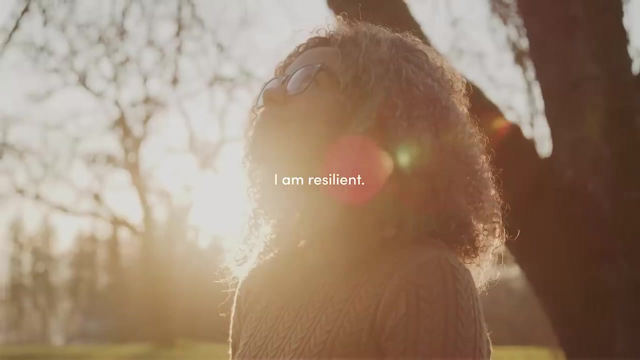 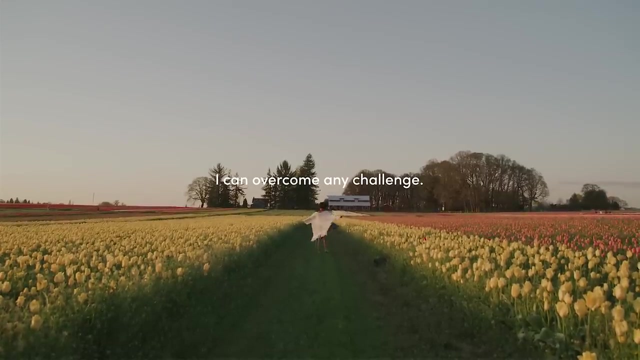 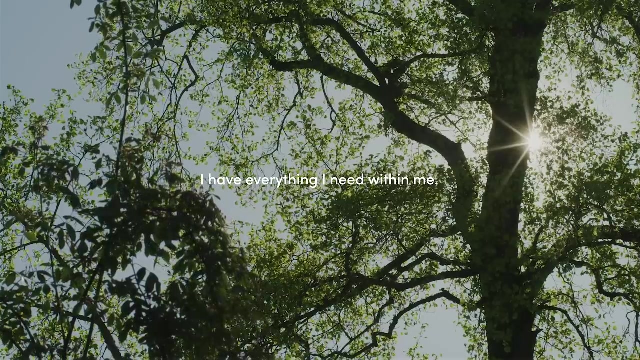 yourself and purpose. I am always growing and evolving. I am always growing and evolving. I am resilient. I am resilient. I can overcome any challenge. I can overcome any challenge. I have everything I need within me. I have everything I need within me. 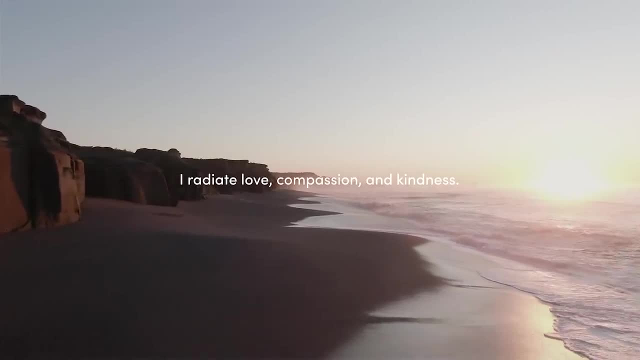 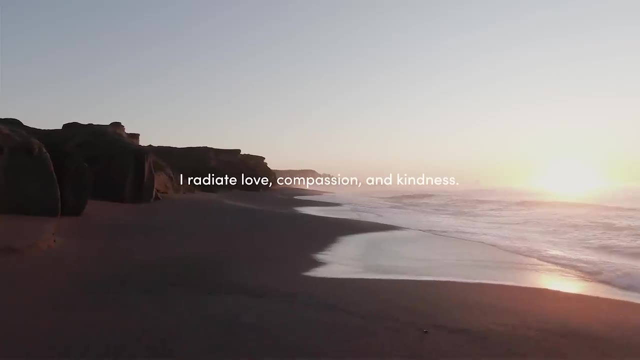 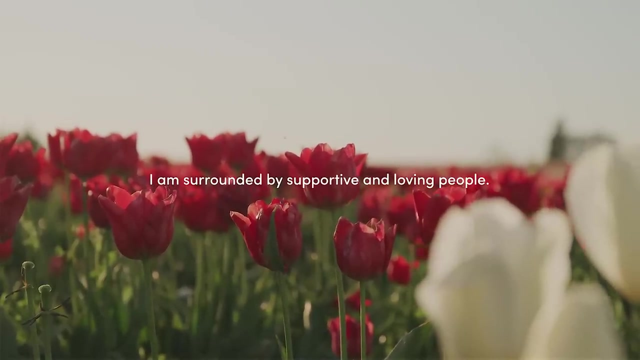 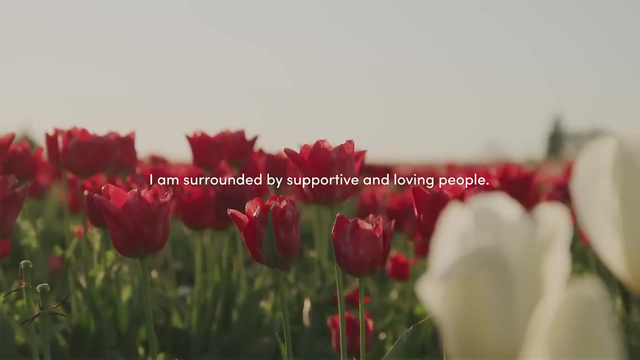 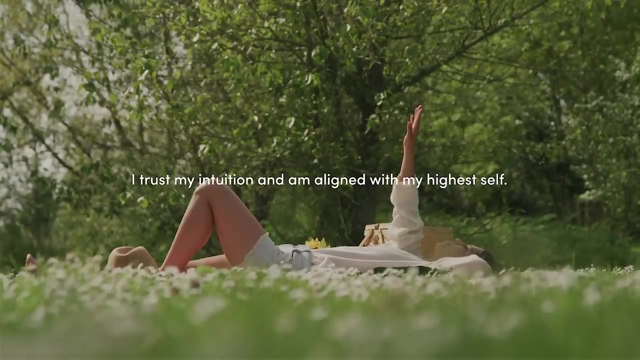 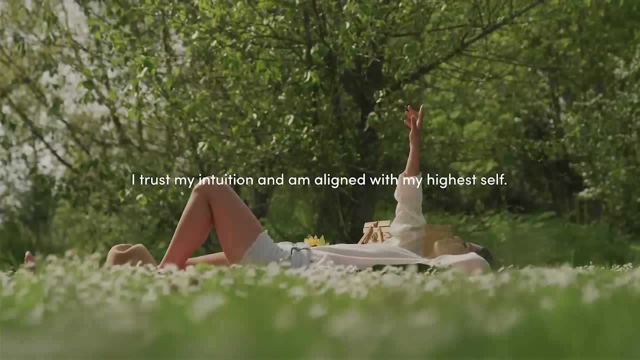 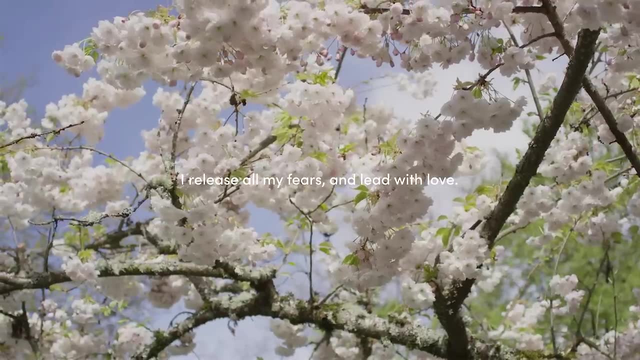 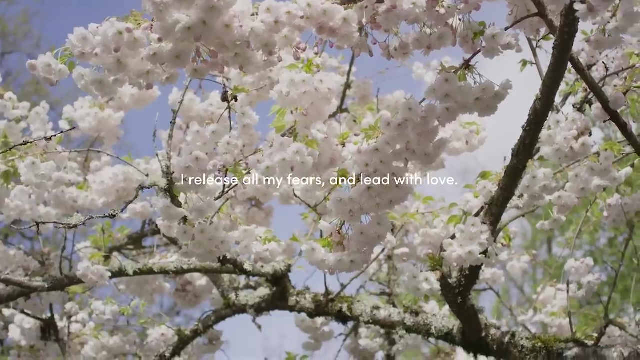 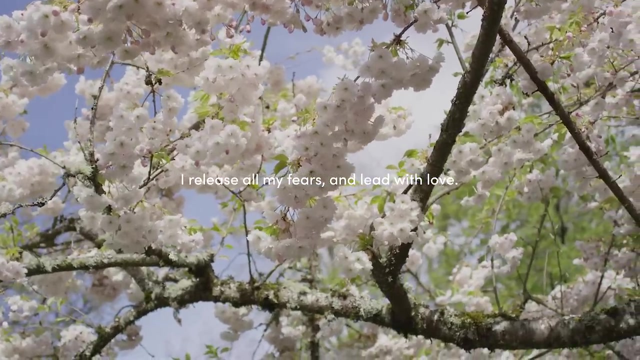 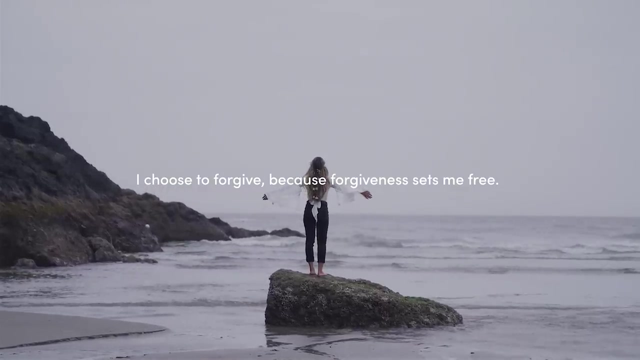 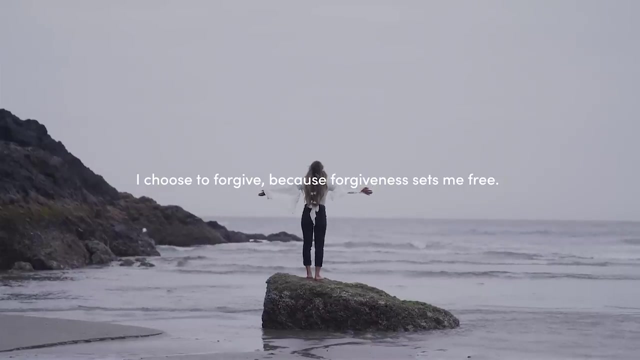 I trust my intuition and am aligned with my highest self. I release all my fears and lead with love. I release all my fears and lead with love. I choose to forgive because forgiveness sets me free. I choose to forgive because forgiveness sets me free. 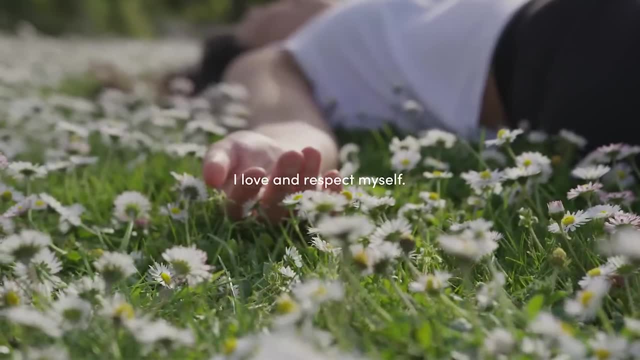 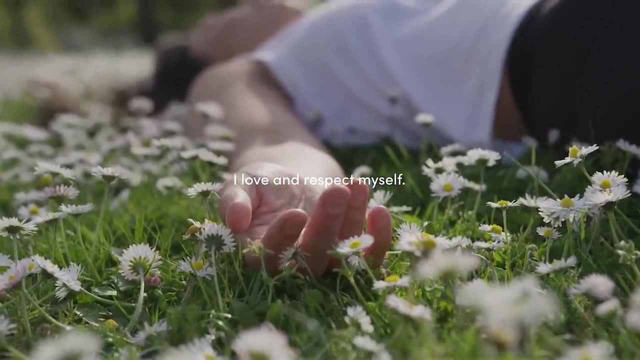 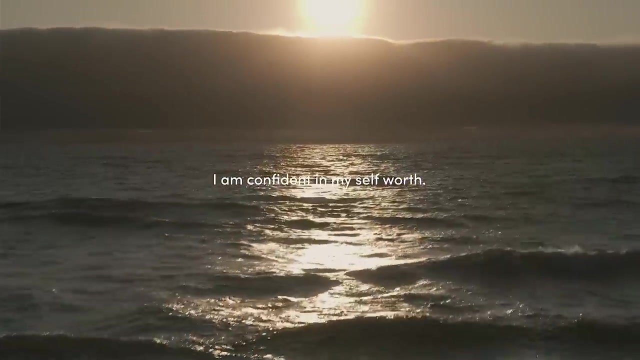 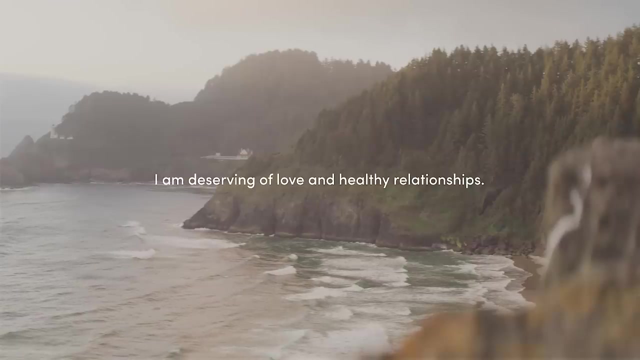 I love and respect myself. I love and respect myself. I am confident in my self-worth. I am confident in my self-worth. I am confident in my self-worth. I am deserving of love and healthy relationships. I am deserving of love and. 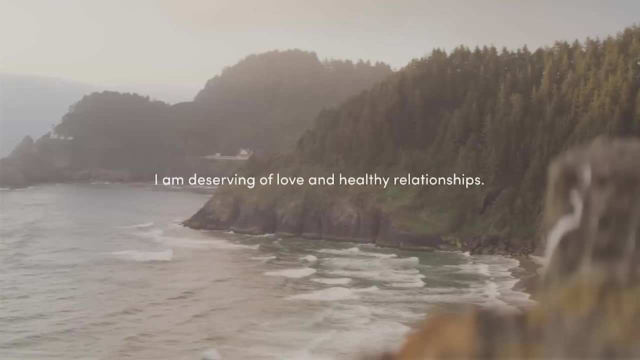 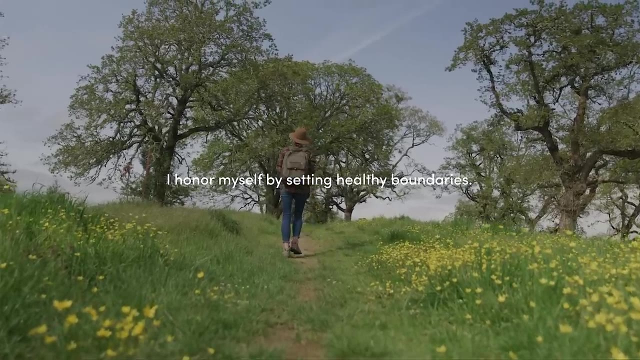 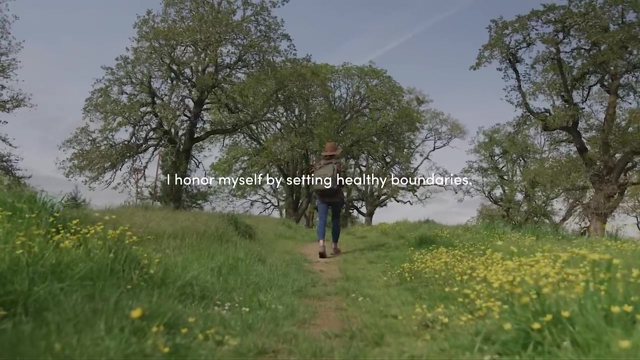 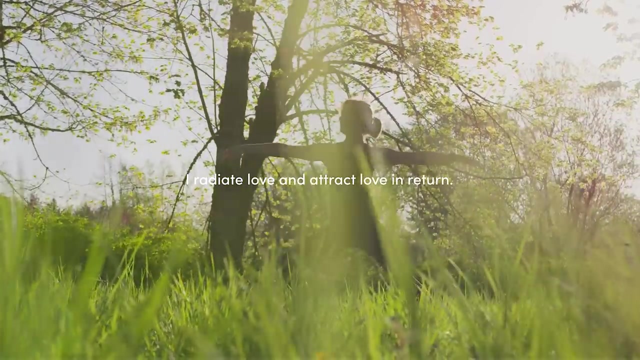 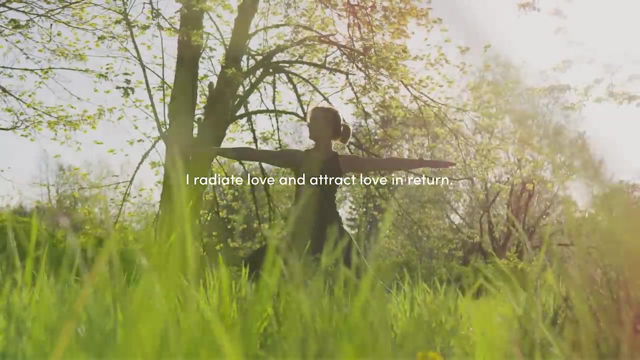 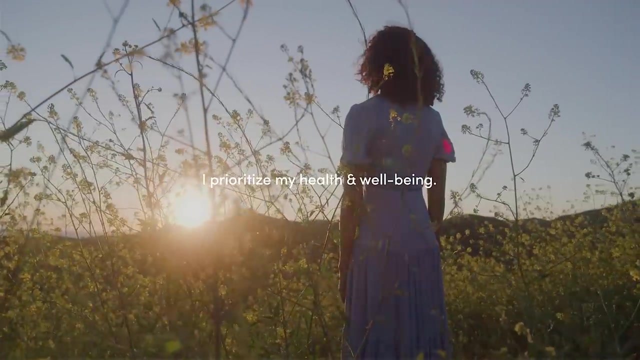 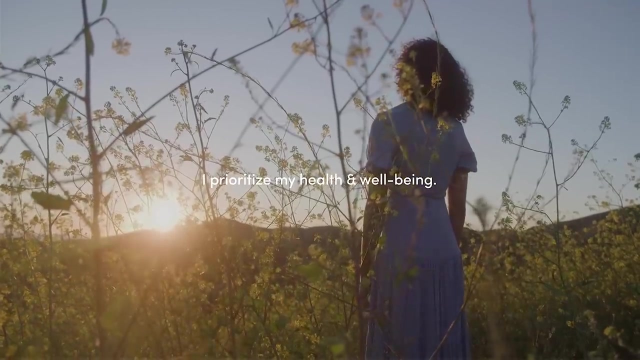 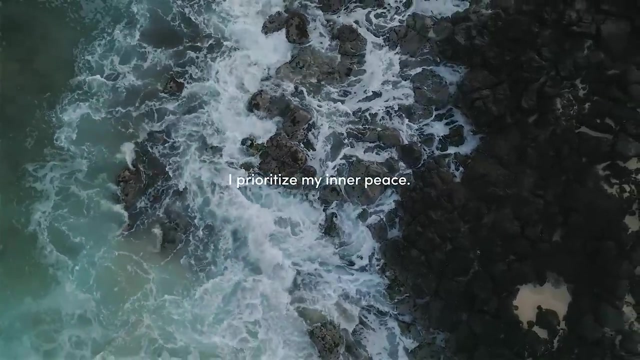 healthy relationships. I honor myself by setting healthy boundaries. I honor myself by setting healthy boundaries. I radiate love and attract love in return. I radiate love and attract love in return. I prioritize my health and well-being. I prioritize my health and well-being. I health and well-being. i prioritize my inner peace. i prioritize my inner peace. 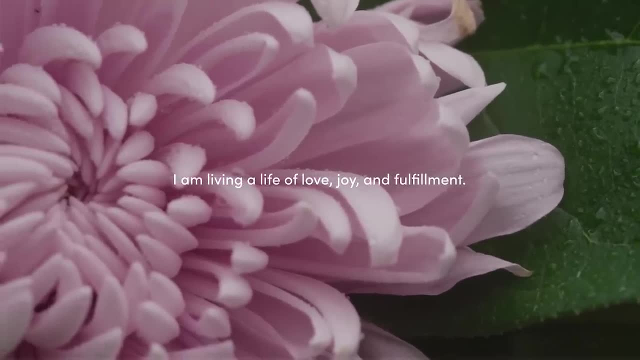 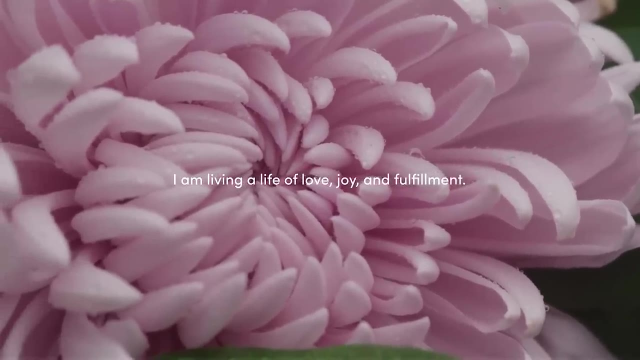 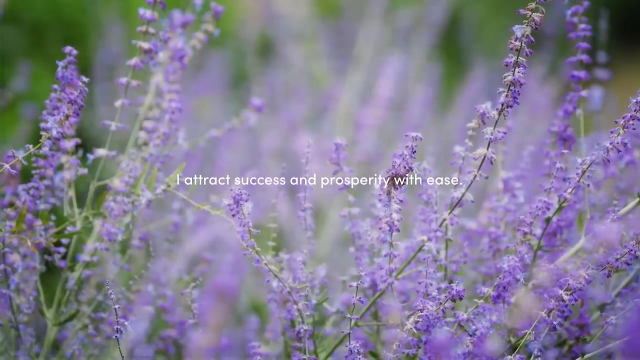 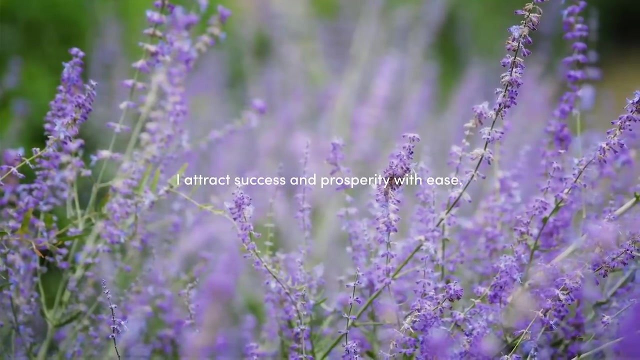 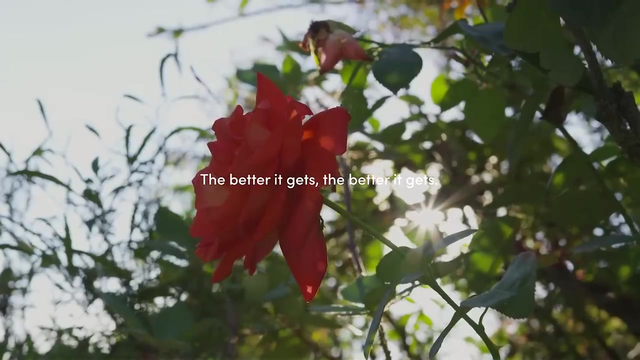 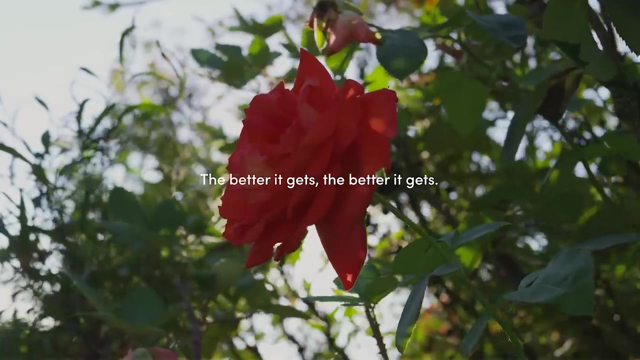 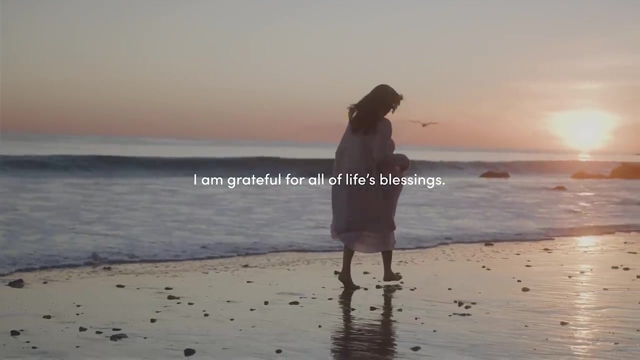 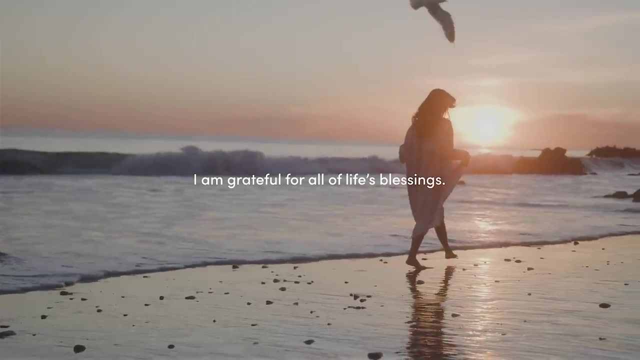 i am living a life of love, joy and fulfillment. i am living a life of love, joy and fulfillment. i attract success and prosperity with ease. i attract success and prosperity with ease. the better it gets, the better it gets, the better it gets. I am grateful for all of life's blessings. 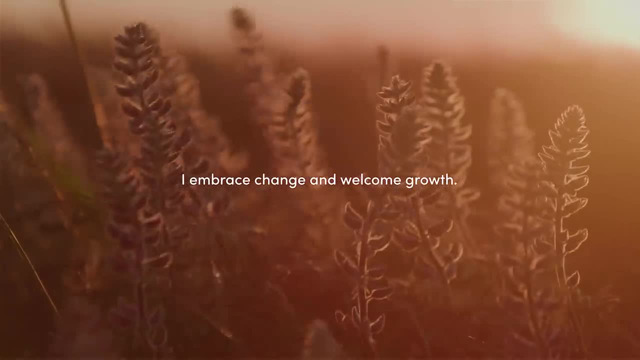 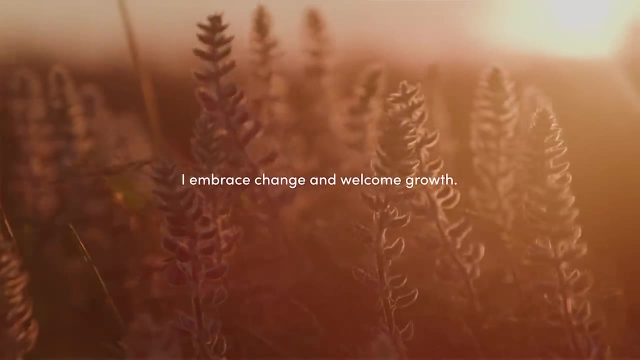 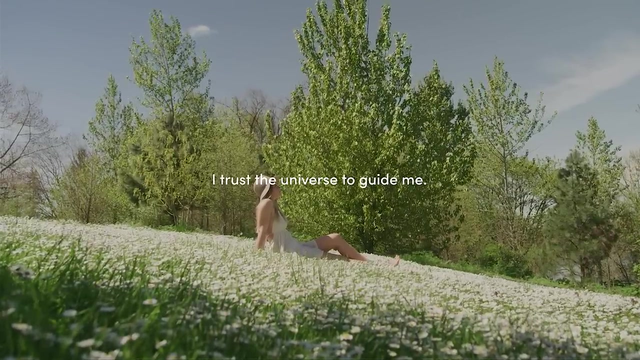 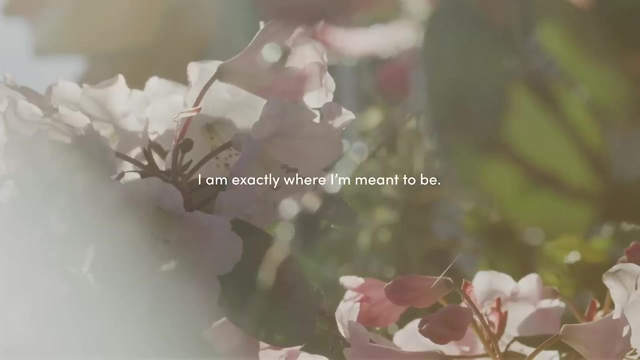 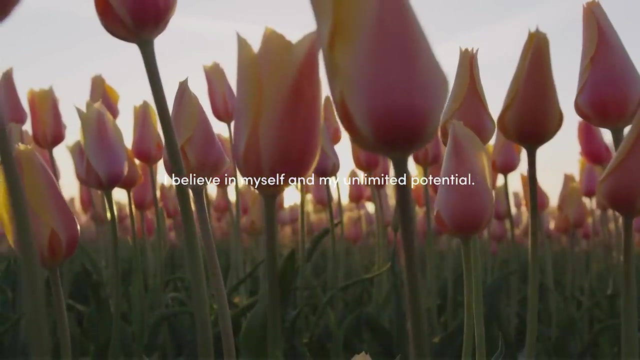 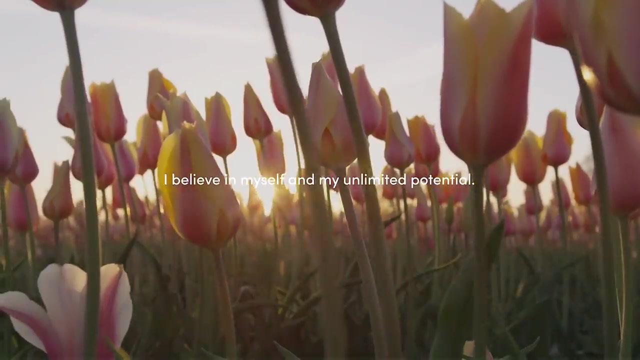 I embrace change and welcome growth. I trust the universe to guide me. I am exactly where I'm meant to be. I believe in myself and my unlimited potential. I believe in myself and my unlimited potential. I believe in myself and my unlimited potential. 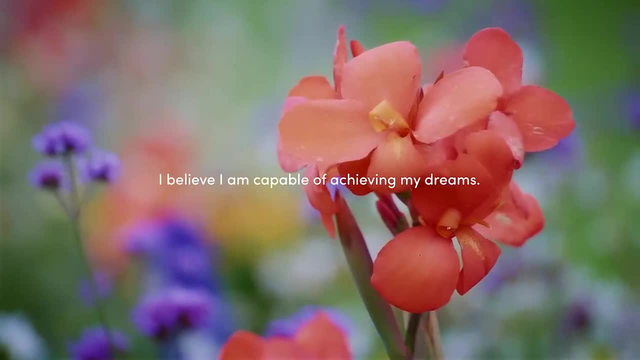 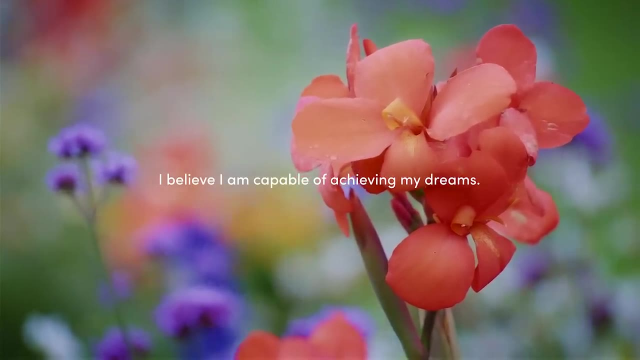 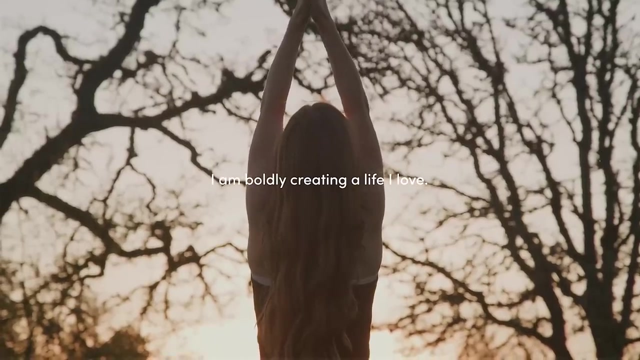 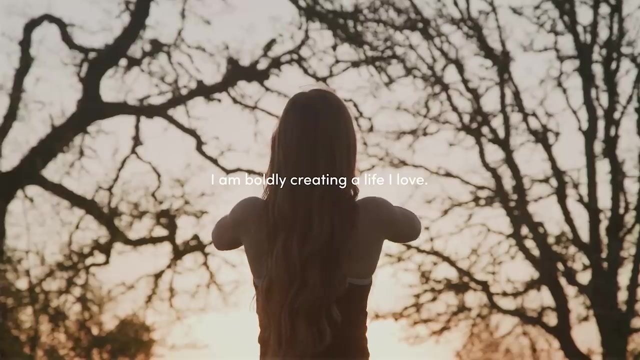 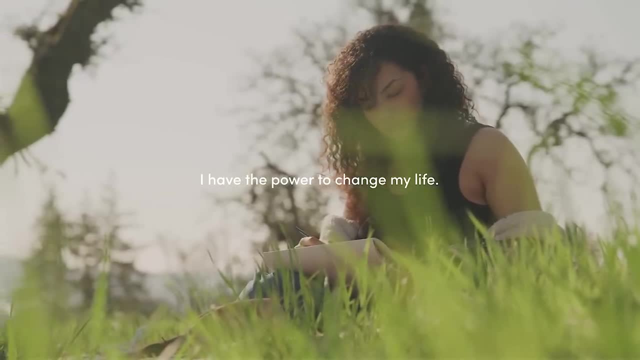 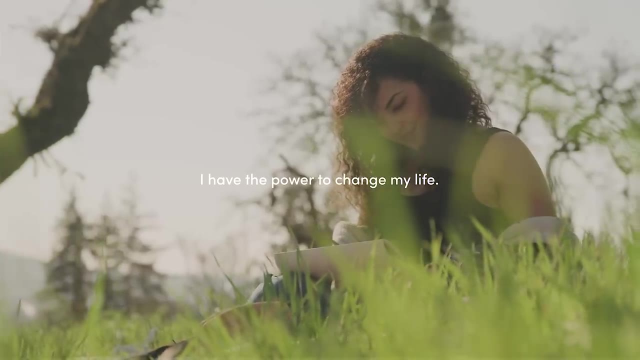 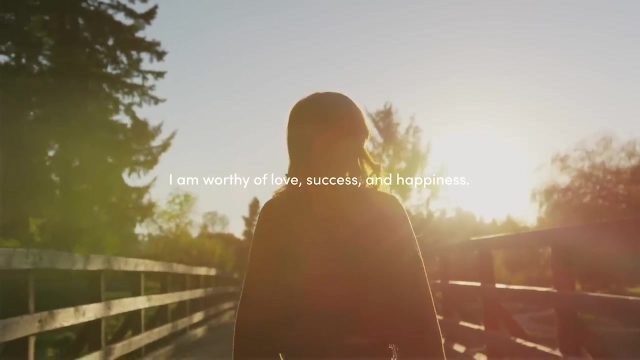 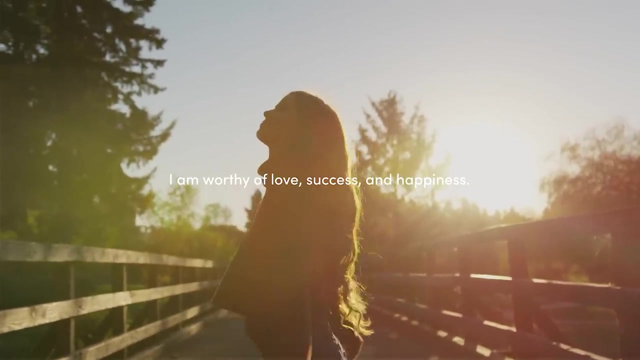 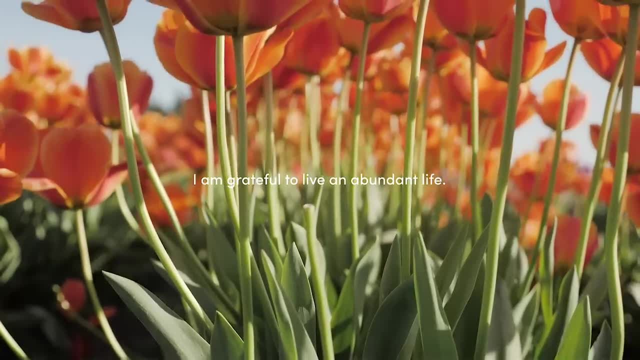 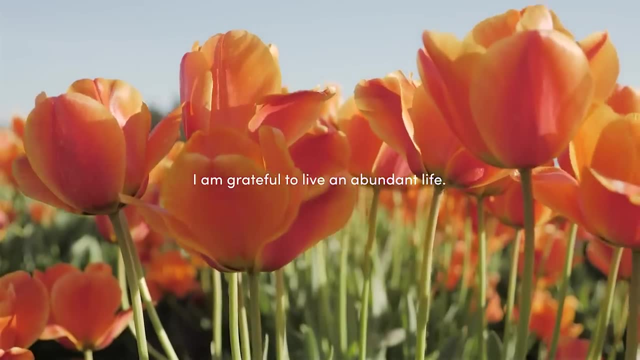 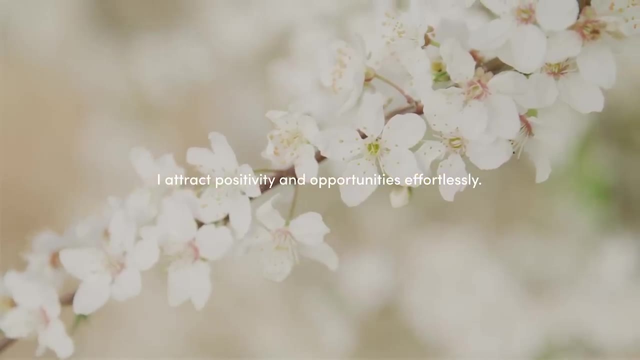 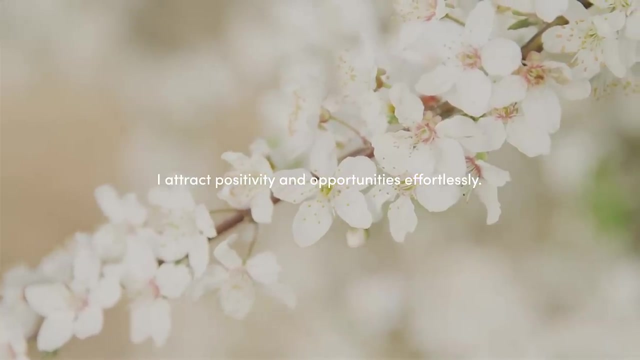 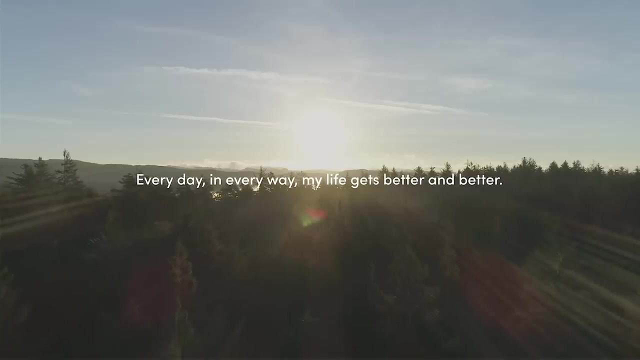 I am worthy of love, success and happiness. I am grateful to live an abundant life. I attract positivity and opportunities effortlessly and I feel so touched. Every day, in every way, my life gets better and better. Every day, in every way, my life gets better and better. 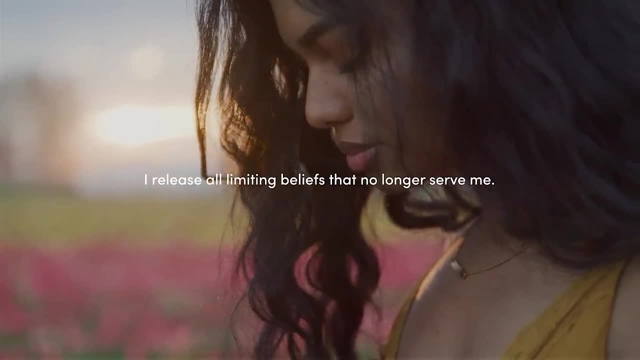 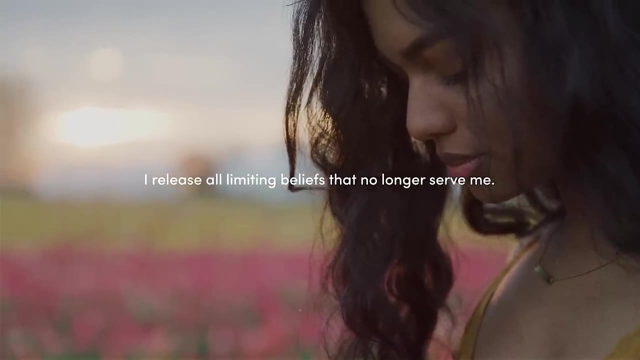 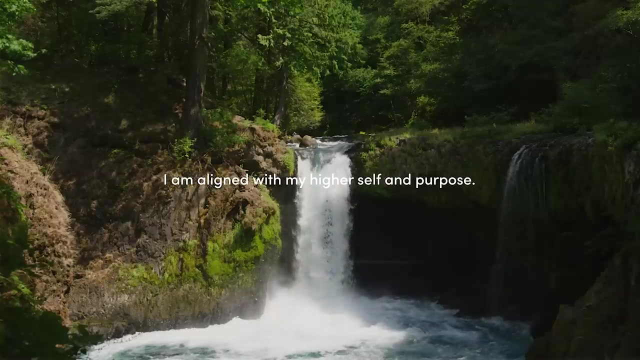 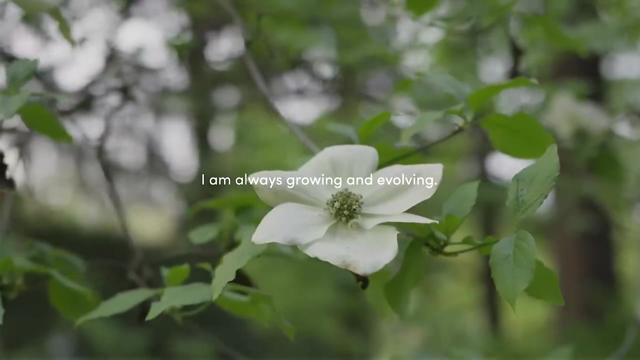 I release all limiting beliefs that no longer serve me. I release all limiting beliefs that no longer serve me. I am aligned with my higher self and purpose. I am aligned with my higher self and purpose. I am always growing and evolving. I am always growing and evolving. 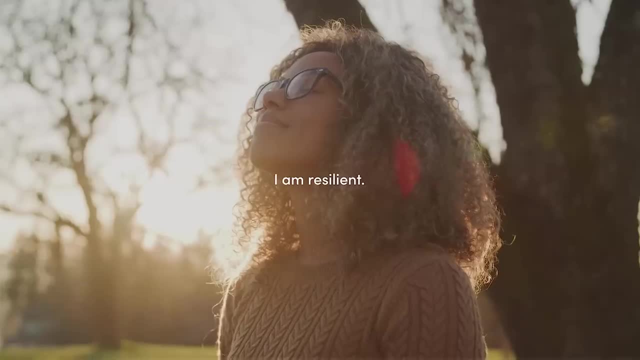 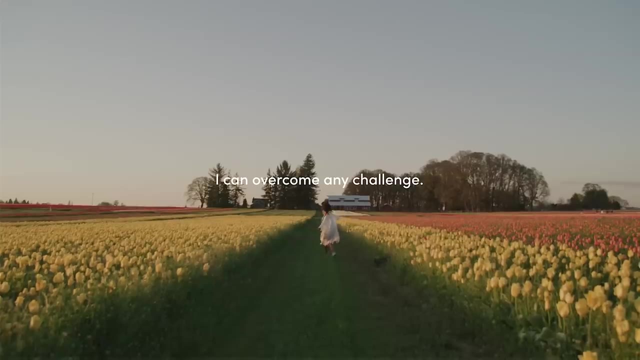 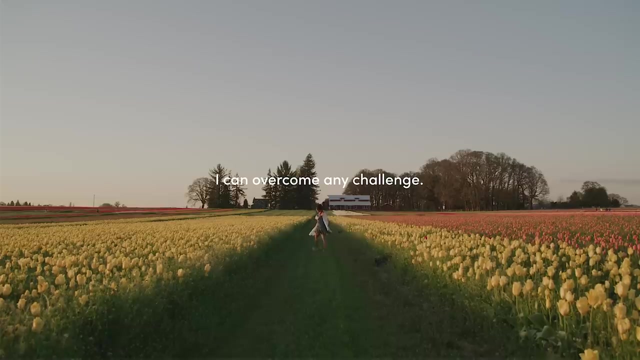 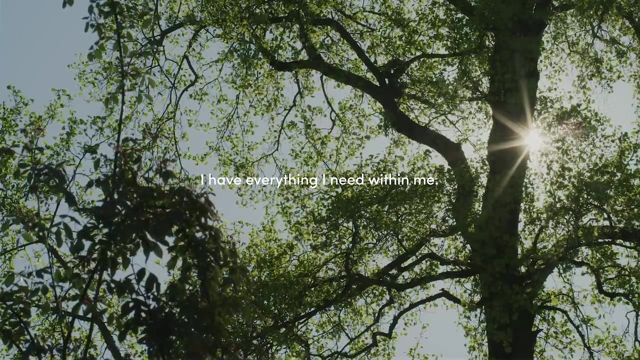 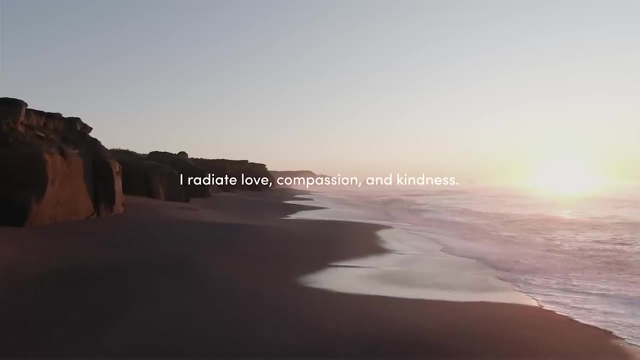 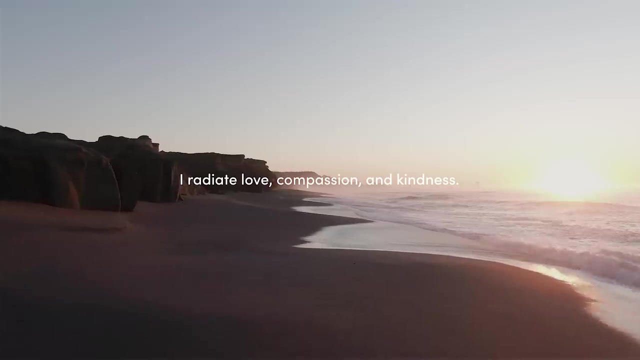 I am resilient. I am resilient, I can overcome any challenge. I can overcome any challenge. I have everything I need within me. I have everything I need within me. I radiate love, compassion and kindness. I radiate love, compassion and kindness. 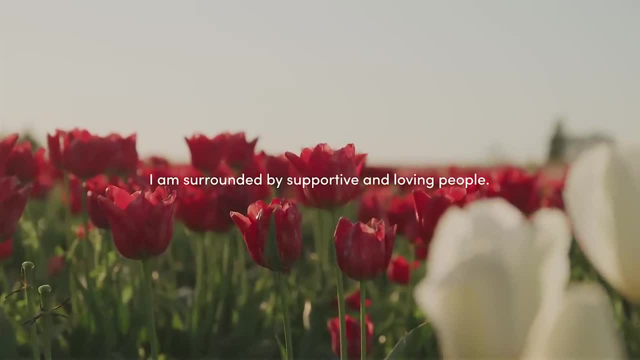 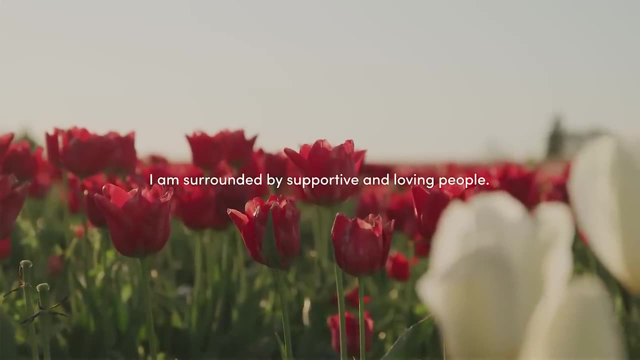 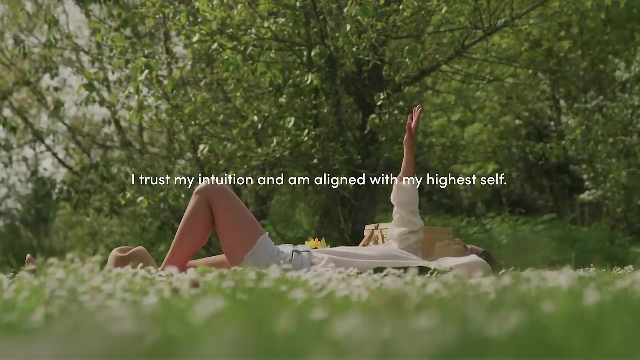 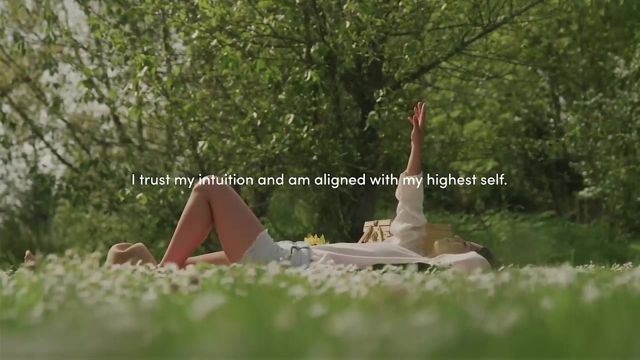 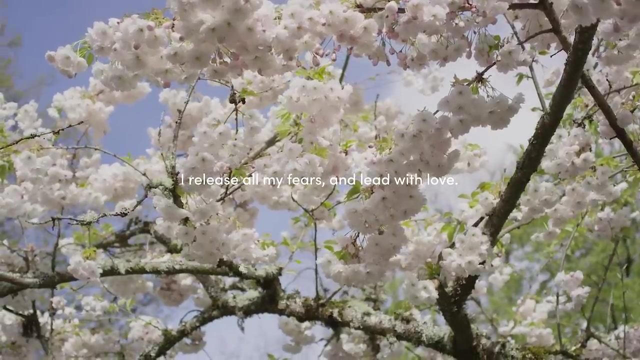 I am surrounded by supportive and loving people. I am surrounded by supportive and loving people. I trust my intuition and am aligned with my highest self. I trust my intuition and I'm aligned with my highest self. I release all my fears and lead with love. I release all my fears and 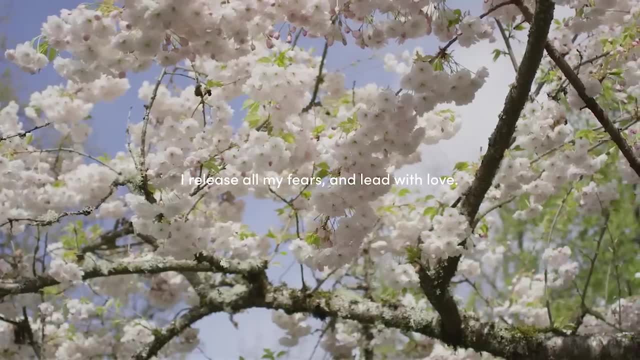 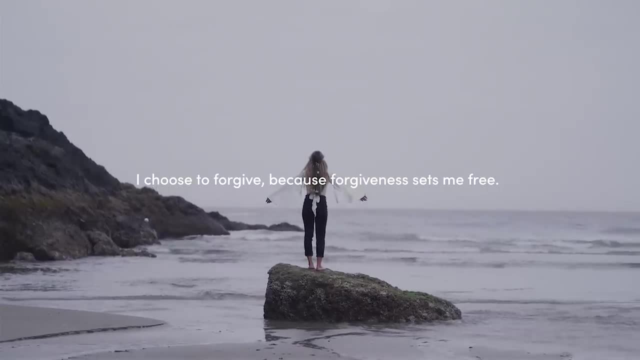 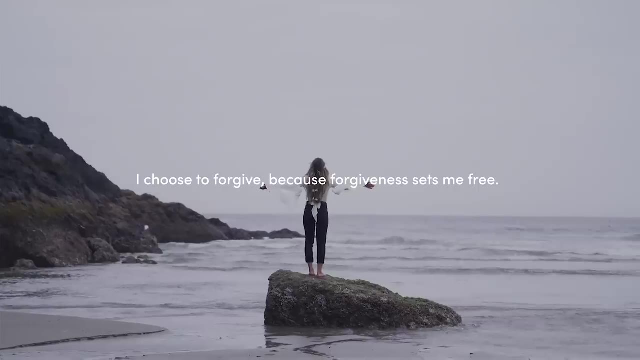 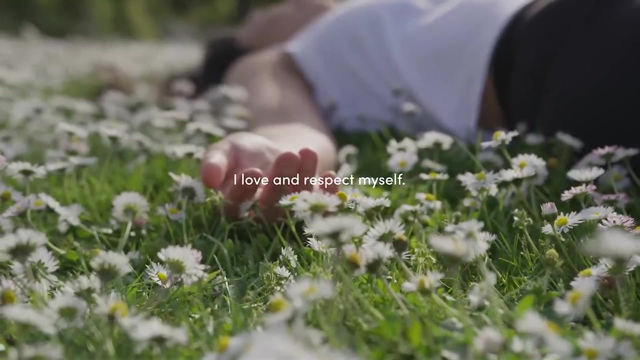 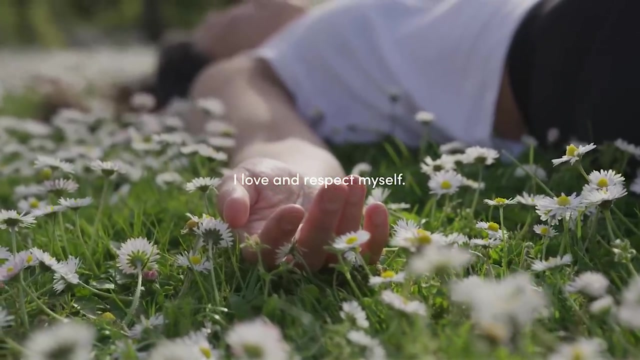 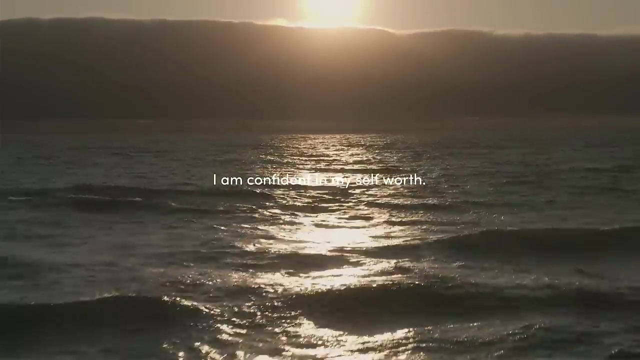 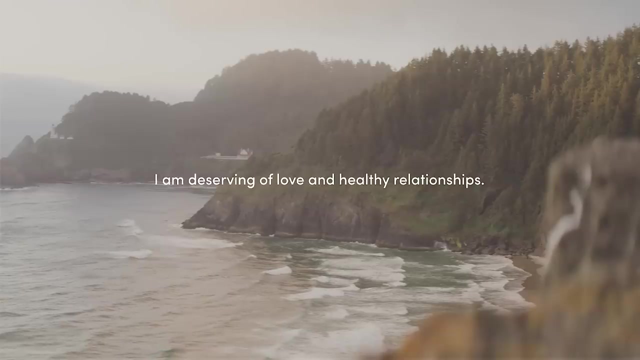 and lead with love. I choose to forgive because forgiveness sets me free. I choose to forgive because forgiveness sets me free. I love and respect myself. I am confident in my self-worth. I am deserving of love and healthy relationships. I am deserving of love. 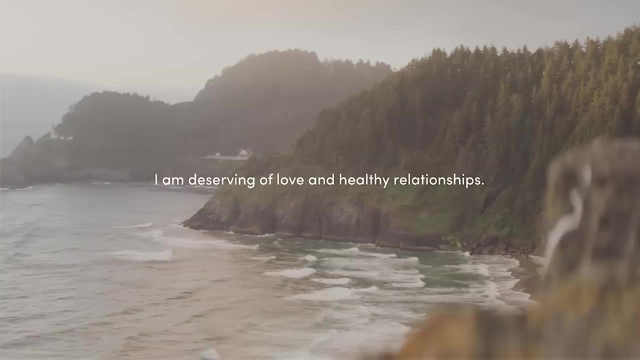 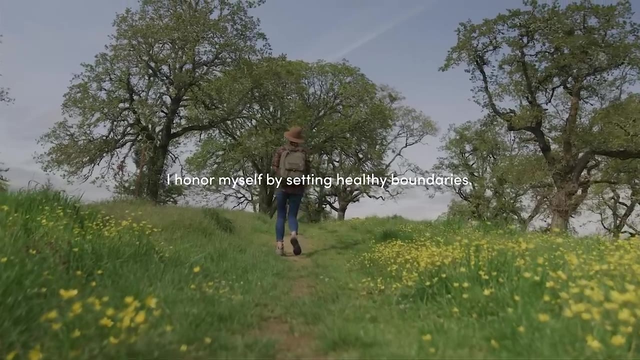 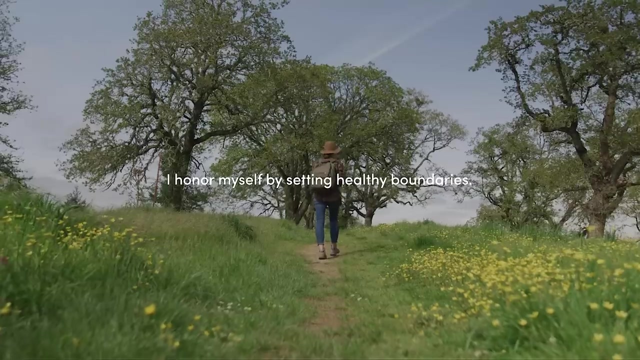 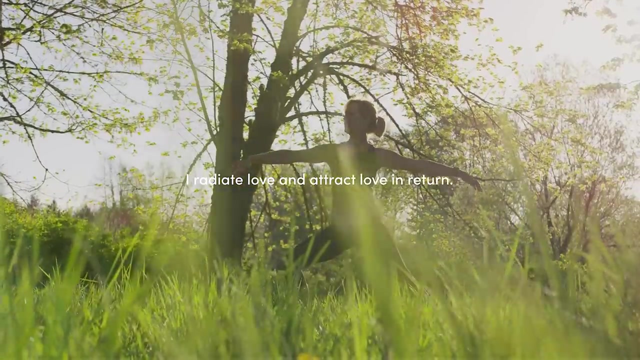 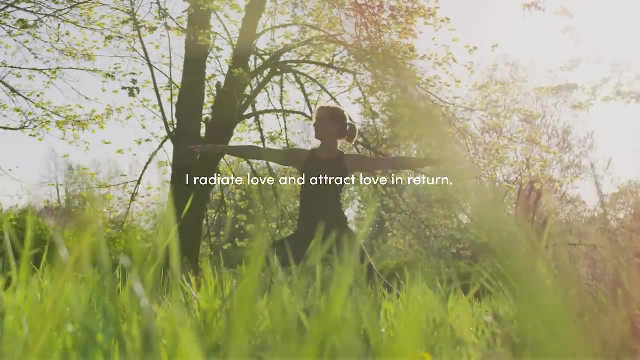 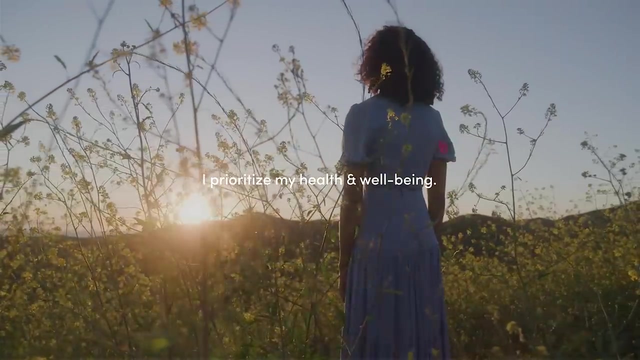 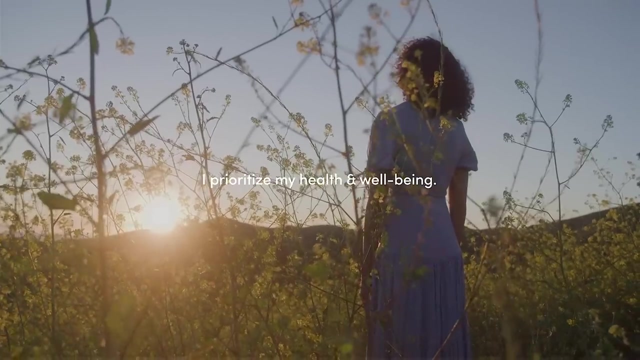 I am deserving of love and healthy relationships. relationships. I honor myself by setting healthy boundaries. I honor myself by setting healthy boundaries. I radiate love and attract love in return. I radiate love and attract love in return. I prioritize my health and well-being. I prioritize my health and well-being. 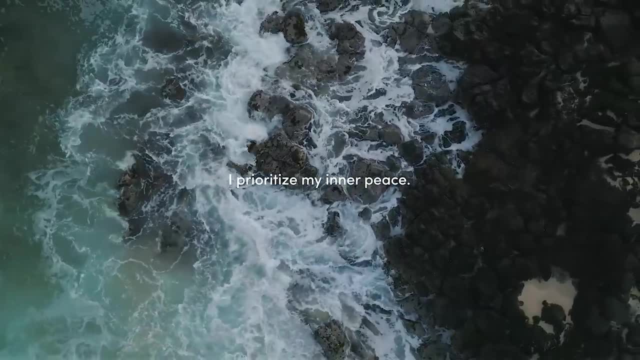 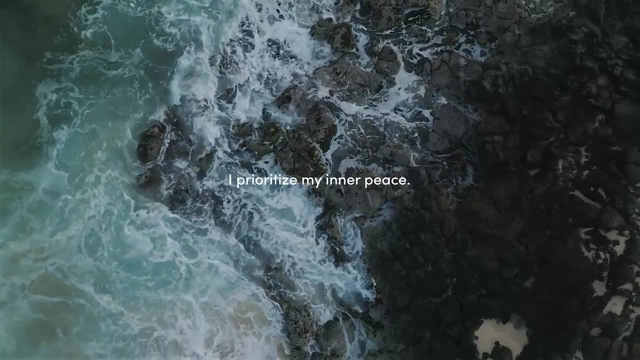 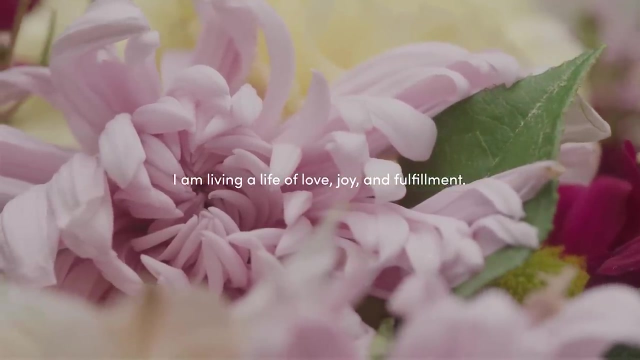 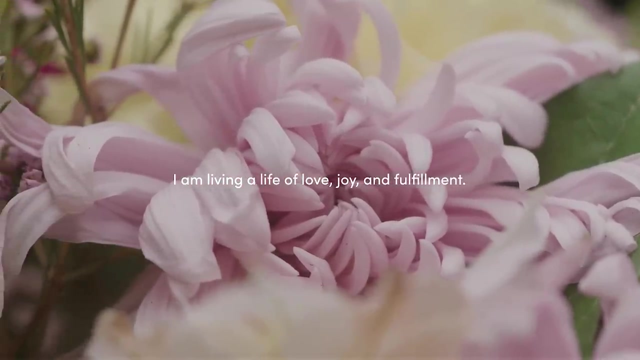 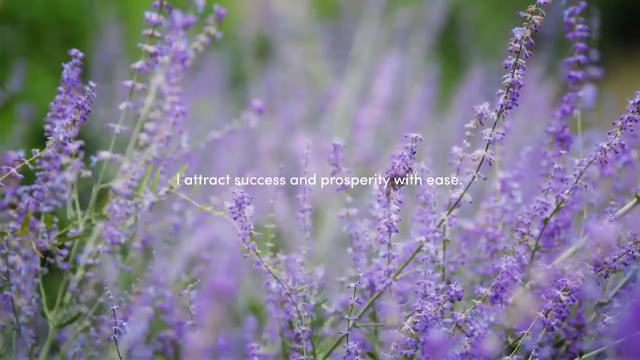 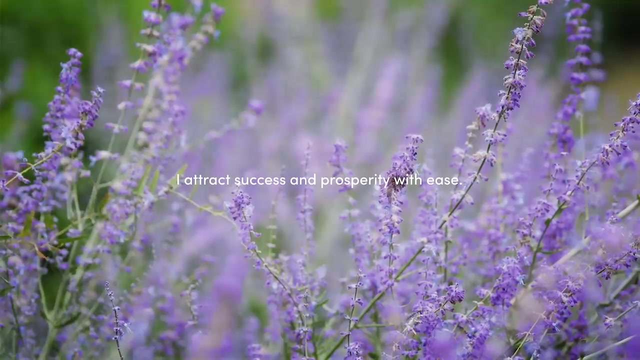 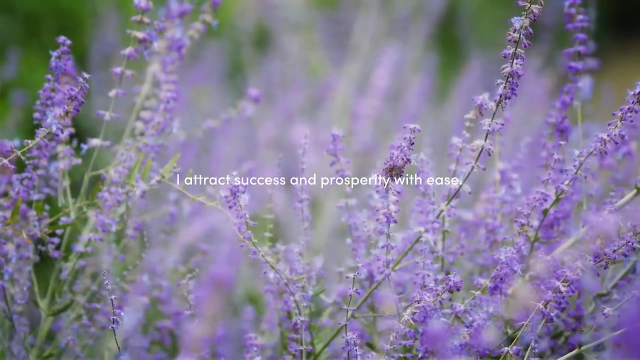 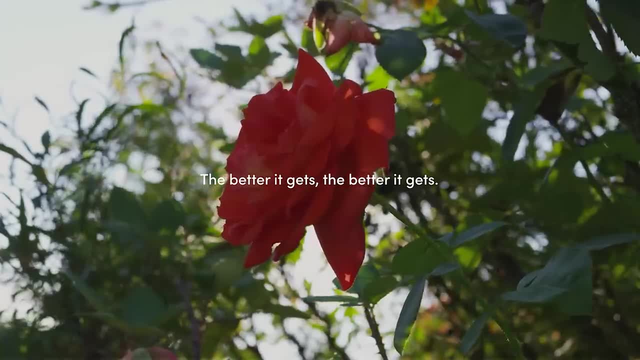 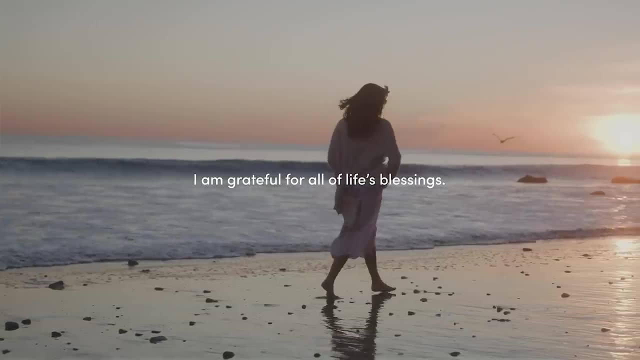 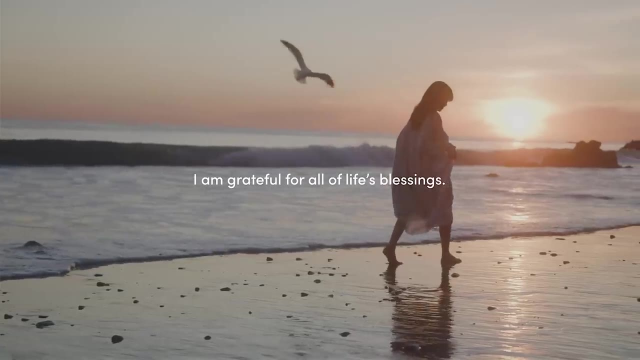 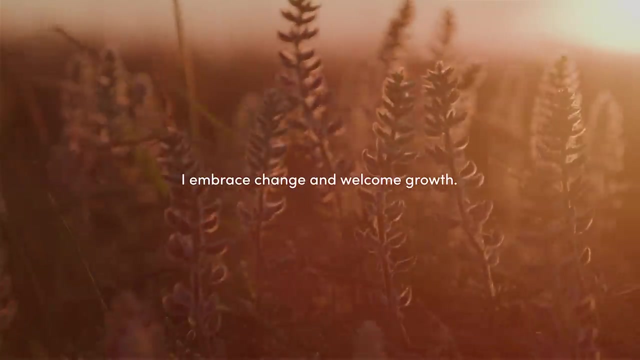 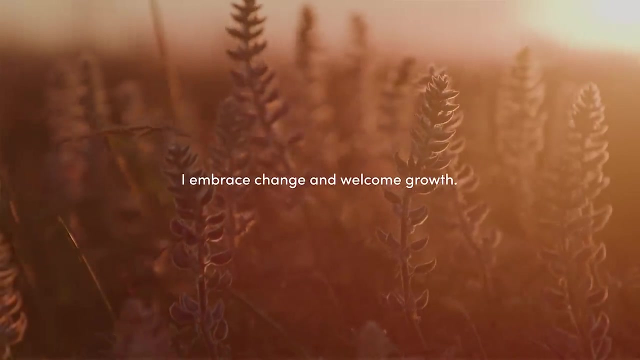 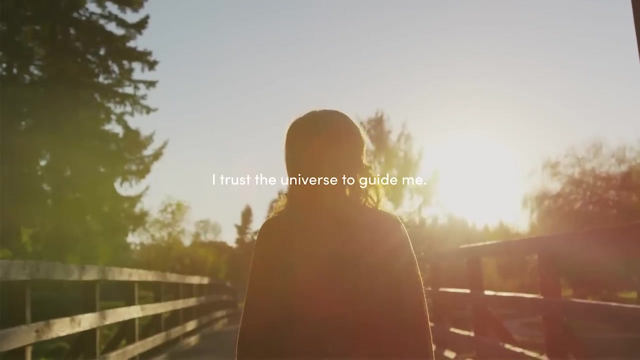 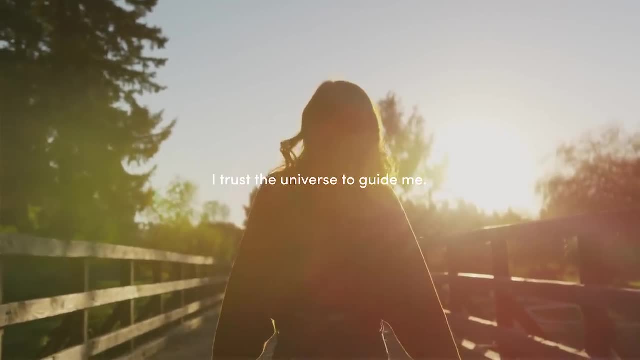 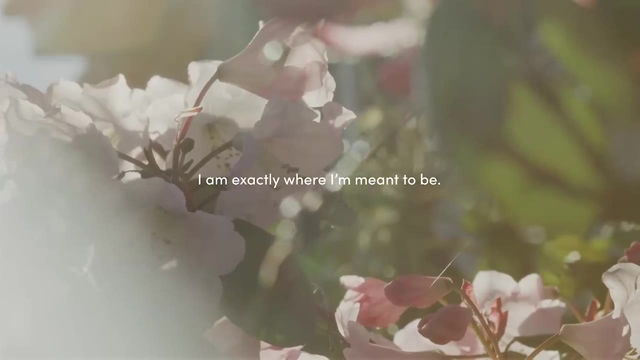 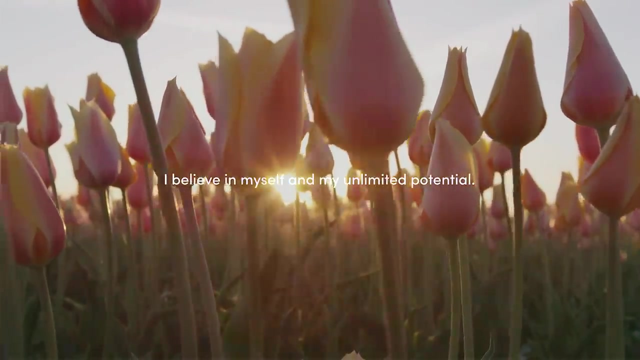 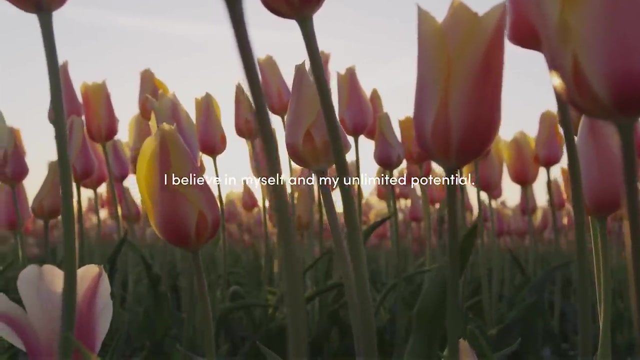 I trust the universe to guide me. Trust the universe to guide me. I am exactly where I'm meant to be. I am exactly where I'm meant to be. I believe in myself and my unlimited potential. I believe in myself and my unlimited potential.